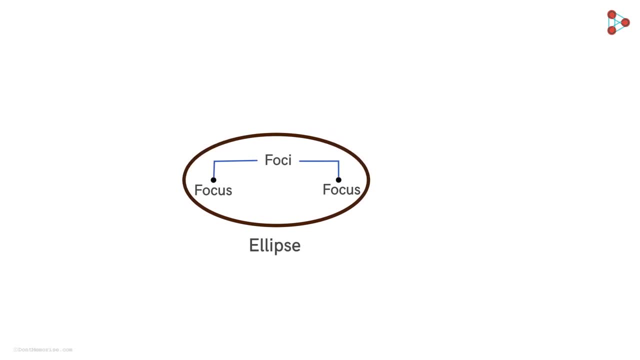 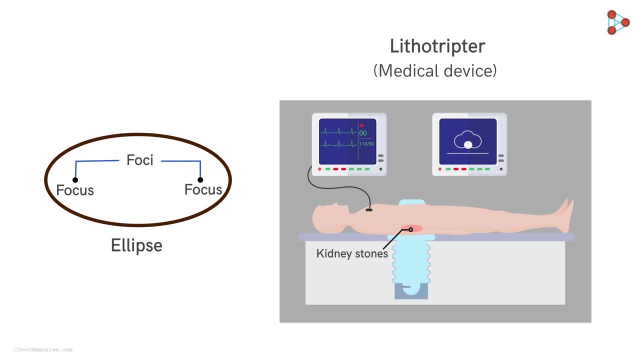 Elliptical shapes even play a role in a medical device called the lithotryptor. Due to its reflective property, it is used to break the kidney stones. High-frequency shock waves are generated at one focus of the elliptical shaped reflector. 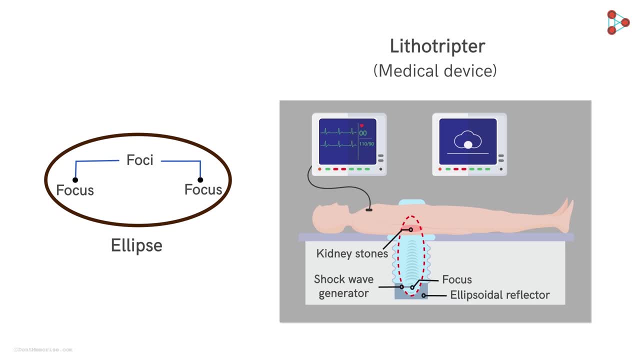 and at the same time, they are used to break the kidney stones, Which gets concentrated at another focus point where the kidney stones are positioned, And this helps in breaking the kidney stones. There is so much more that can be done with an elliptical shape. 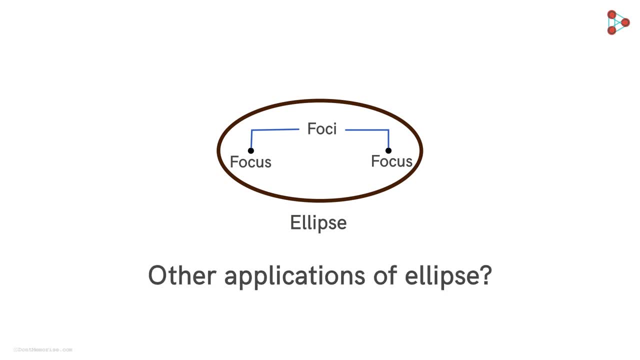 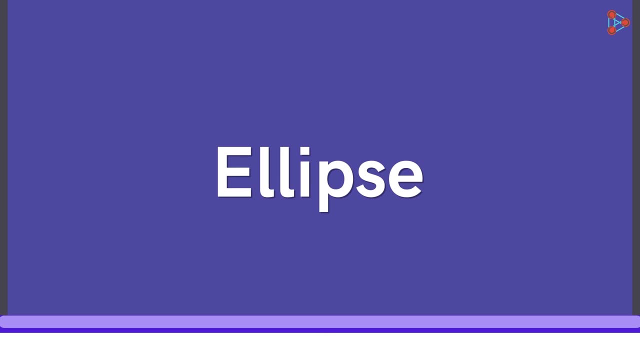 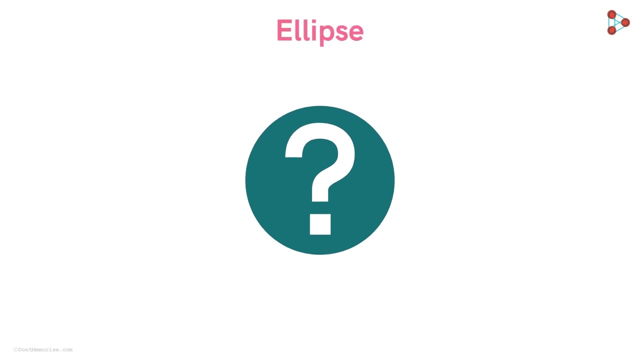 Can you explore other applications of this shape and tell us in the comments section below? In the next part, let's understand what exactly an ellipse is. How do we understand the shape of an ellipse? Suppose we have two points in a plane. We name this point as F1 and this point as F2.. 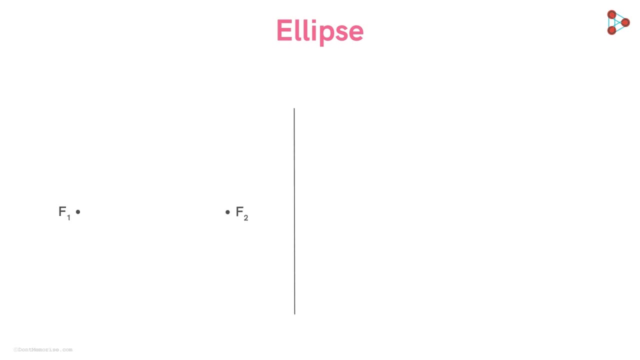 Now consider a special set of points on the same plane. They are placed such that their sum of the distances from these two points is constant. Let me explain. Suppose we take a point here, Let's name it A. Now let's say the sum of its distances from point F1 and point F2. 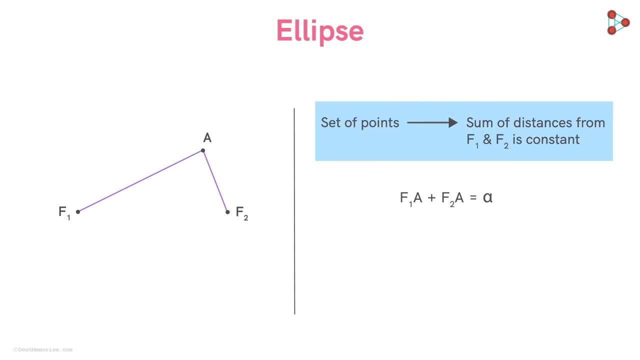 is some number, alpha. Now consider all such points whose sum of the distance from these two points is exactly equal to alpha. Are there any such points? Yes, there are many more. The collection of all such points is called an ellipse. Let's say we take a point B on the ellipse. 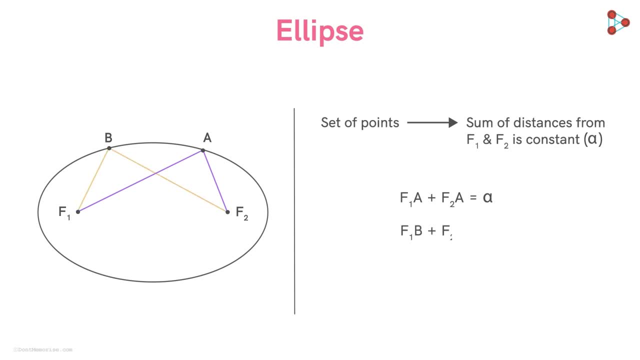 Then the sum of its distances from the points F1 and F2 will be alpha. Let's take another point C. here Again, the sum of its distances from the points F1 and F2 will be alpha. So we see that the ellipse is a collection of all points in a plane. 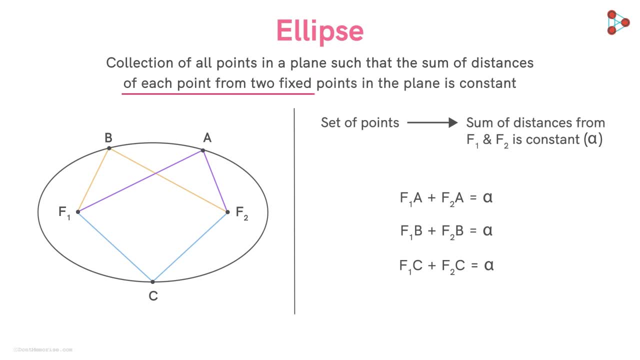 such that their sum of distances from the two fixed points in the plane is constant. Each fixed point, F1 and F2, is called the focus of the ellipse, And together they are called the foci of the ellipse. Here we took the constant to be alpha.